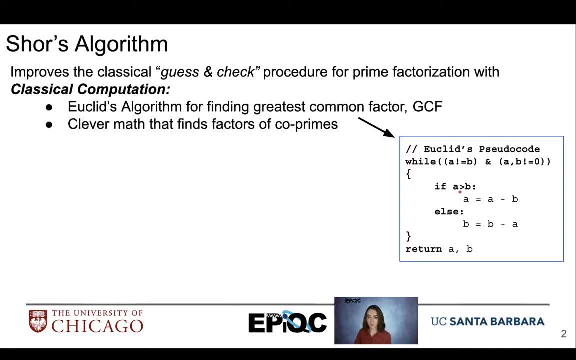 factor between them. So we first see which number is larger, A or B, and we subtract the smaller from the larger. We continue this procedure until A and B are equal, or either A or B is equal to zero. Then we know that we've found our greatest common factor. For the clever math that helps us find 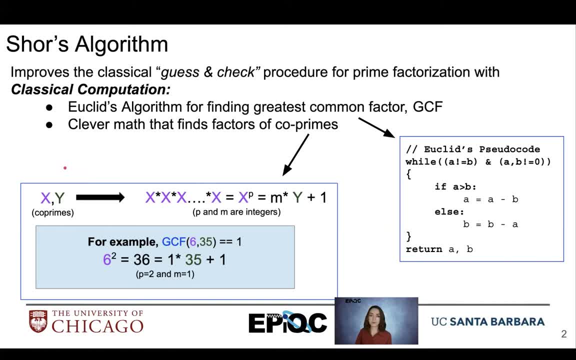 factors of co-primes. we take two co-prime values, So here we'll use X and Y and we raise X to some value P that allows us to find a multiple of Y plus one. So for example, we have two co-primes. 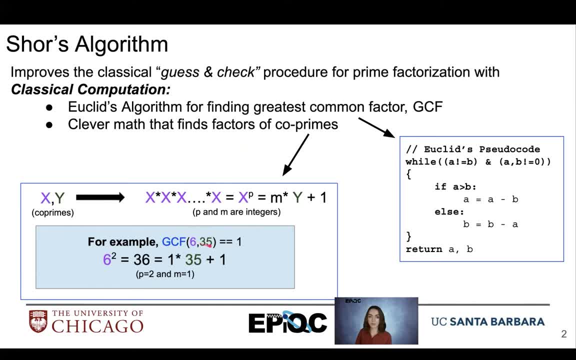 6 and 35.. We know they're co-primes because their greatest common factor is one And we raise 6 to the 2 to get 36, or 1 times 35 plus 1.. So in this example, we know that P is equal to 2 and N is equal to 1.. Now, as a note, co-prime values. 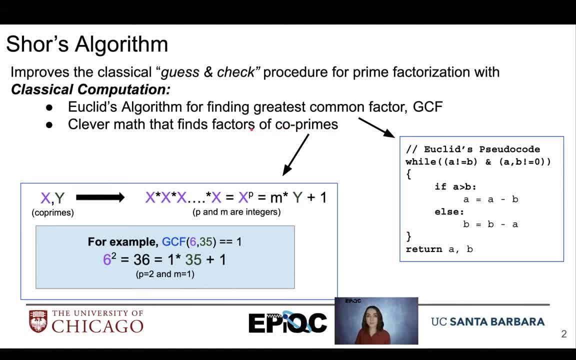 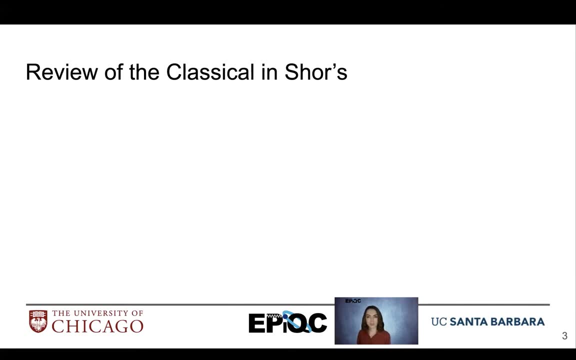 don't necessarily have to be primes themselves. They just have to be two values where their greatest common factor is 1.. The quantum computation in Schwarz's algorithm involve routines that quickly find P. We're going to look at that in a moment. Let's review the classical components of Schwarz's algorithm. We have a large number N, and we hope 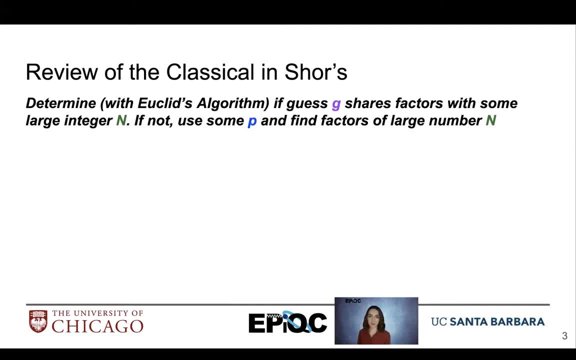 to factor it. So we first make a guess of the factor and we'll call that G. We'll use Euclid's algorithm to determine if G shares factors with N. If we find that G shares a factor with N, we're done. That's highly unlikely though, So if not, we are going to find some P to help us find factors. 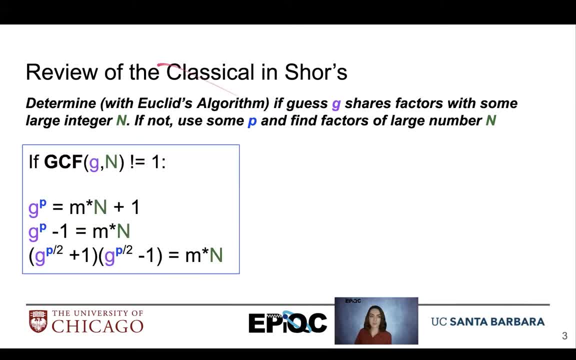 of that large number, N. So we'll look at this. So if the greatest common factor of G and N is not equal to 1, which is highly likely, we are going to have to find some value P that will allow us to find. 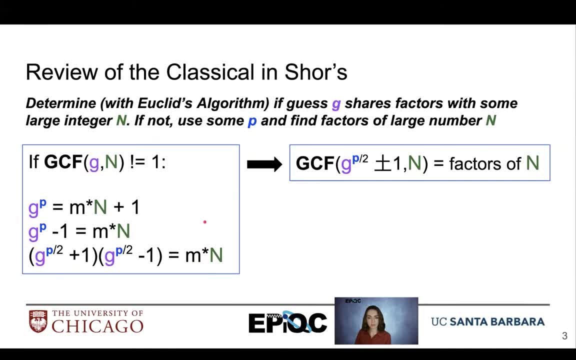 factors of N. We'll cleverly rearrange this information in the following way. so we know that the greatest common factor of G, raised to some P divided by 2 plus or minus 1 and N will equal factors of N. But what is P? 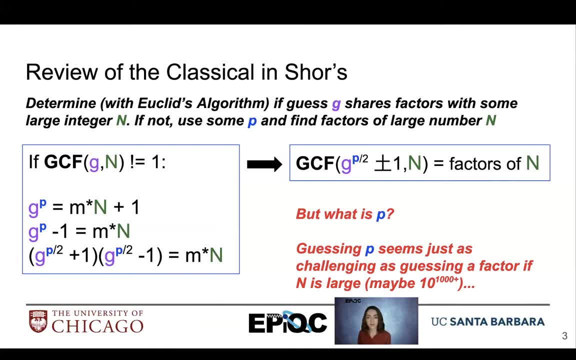 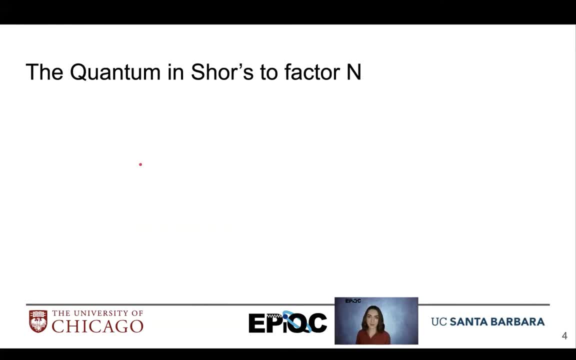 Trying to guess values of P is just as challenging as trying to find a factor, especially if N is very large. This introduces the quantum aspect of Schwarz to factor N. We have this challenge of finding the right P to find G to the P. minus 1 is equal to M times N. But not every P works For. 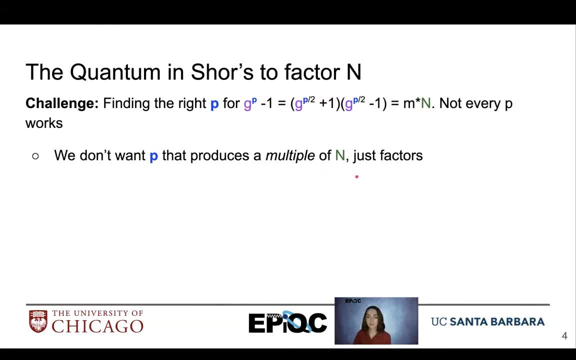 example, we don't want a value of P that produces a multiple of N. We want factors. We also don't want odd values of P, Because that will produce fractions. We need an integer. So, for example, if we had P equal to 1,. 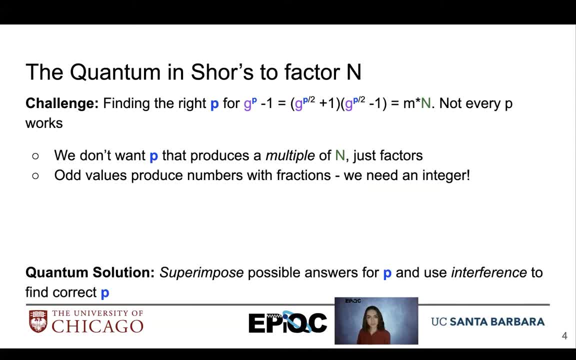 G to the 1 half could give us a fraction. So this introduces our quantum solution. We will superimpose possible values for P and use interference to find the correct value of P very quickly. Before we get to finding P, we need to point out some patterns and numbers. 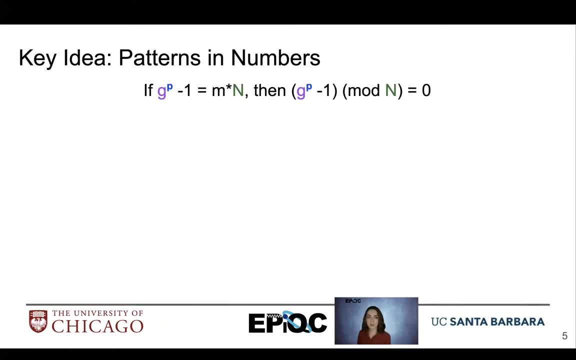 So we have G to the P minus 1 equal to M times N, multiple of N. Then we can make the substitution that G to the P minus 1 modulus N is going to be equal to 0. So let's rearrange that to get G to the P mod N equal to 1.. So as a refresher, 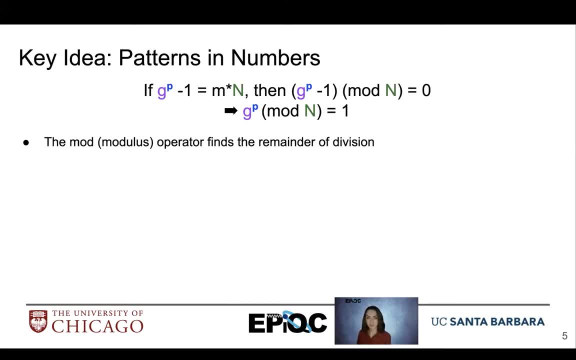 the modulus operation, or mod, finds the remainder of division. So here we have 5. mod 3 is equal to 2.. In the case of our equation above, we see that if we have G to the P minus 1 equals equal to M times N. we know that if we divide this by N, 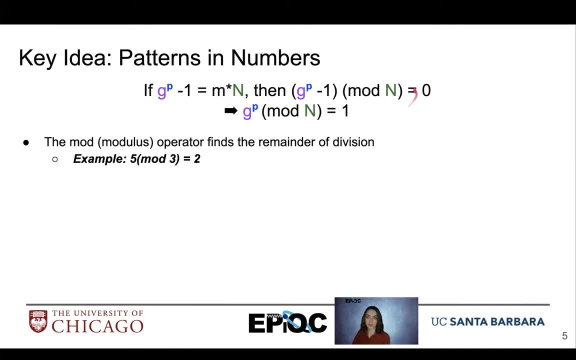 we will get a value M, no remainder. So that's how we get the 0 value here. Something to point out that's very important is that the modulus operation repeats with some certain frequency, with some certain period. So here, if we look at, 0 mod 3 equals 0,. 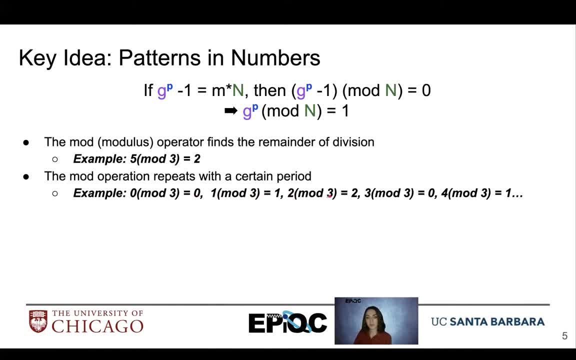 1 mod 3 equals 1, 2 mod 3 equals 2, 3 mod 3 equals 0, we start to see our values appearing again. So we have 0 again and 1 again. Shor's algorithm takes advantage of this and turns a factoring. 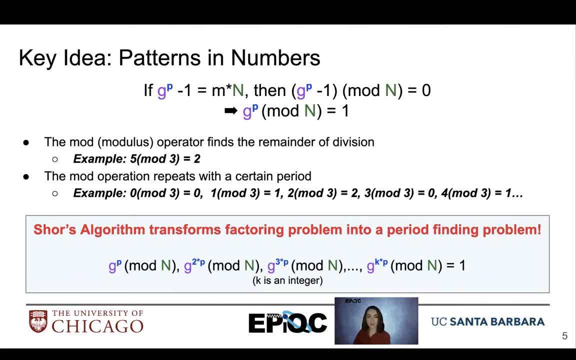 problem into a period finding problem. So if we look at this equation that we just defined up here, we know that if we have P times some multiple value, so here we have G to the P mod N, G to the 2P mod N, G to the 3P mod N, and so on. 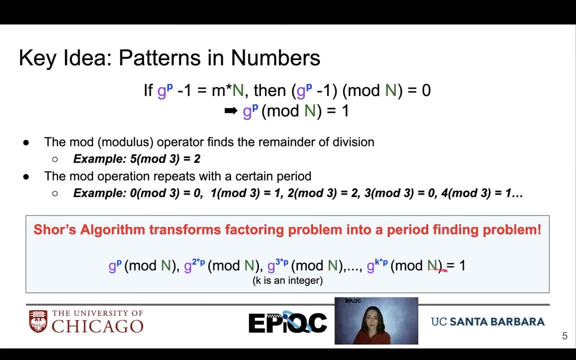 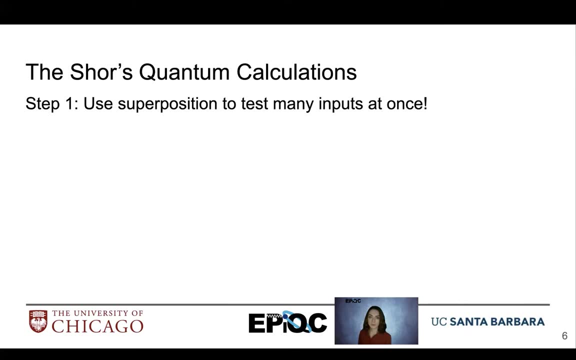 to some value. so some exponent K, that's an integer. we will have all of these equal to 1.. So we have this repetition that we get. that is seen with the modulus operation. With that in mind, we jump to Shor's quantum calculations. We use superposition to test many. 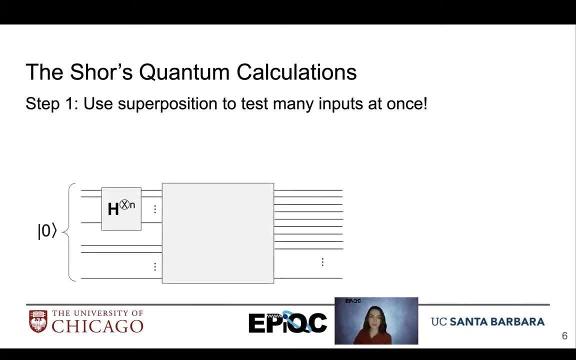 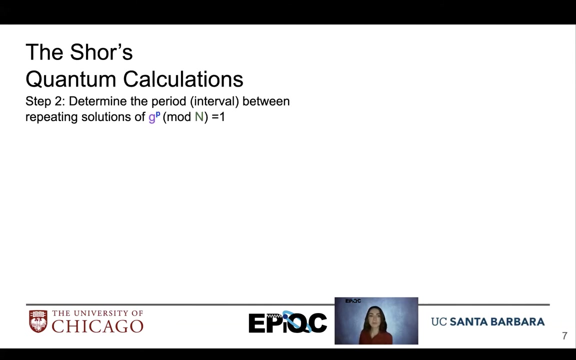 input values at once. So here we can use our Hadamard operation to create a superposition of candidate P values, And then with those superpositions we calculate G to the P mod N. So we calculate all these values here to find a superposition. Now we need to determine the period or interval between repeated solutions of G to the P mod N equal to 1.. Fortunately for us, these have no spherical values: 3 inch to the 3.. If we LEARN how to find x minus h hat, CANNOT guess at all with the sign of H hat. NOT simply call out one of the functions of theяти and NOT called out one of the functions of the other functions importante qu, str, Ethe standard algorithm would in theory generate a new 0 mod N, which is happening with G to the P mod N equal to 1.. 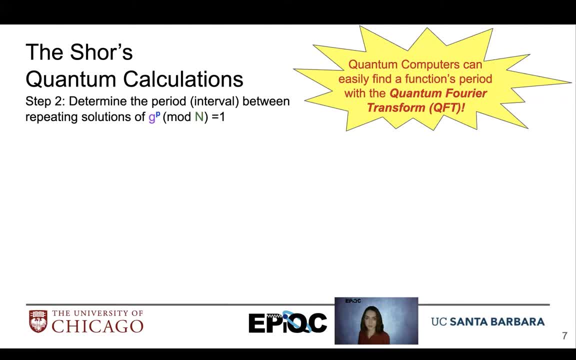 one. Fortunately for us, the quantum Fourier transform, or QFT, can easily find its functions period quickly and efficiently. We're not going to go into depth about the QFT, but I'd highly recommend looking at more information about it. The circuit structure is very well known and 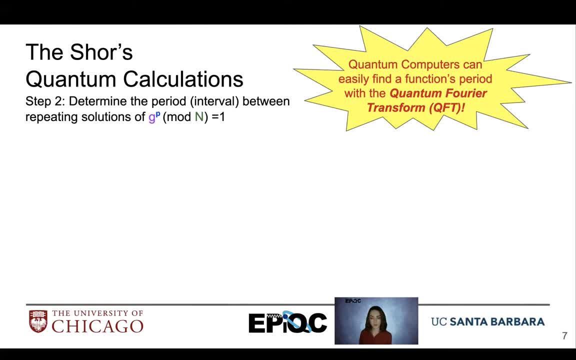 clearly defined, so it's a building block for many popular quantum algorithms. So here we have our first part of our quantum circuit, our superposition, our calculation of g to the p mod n, and then we use the QFT to help us find the interval at which the answer of 1 reappears. 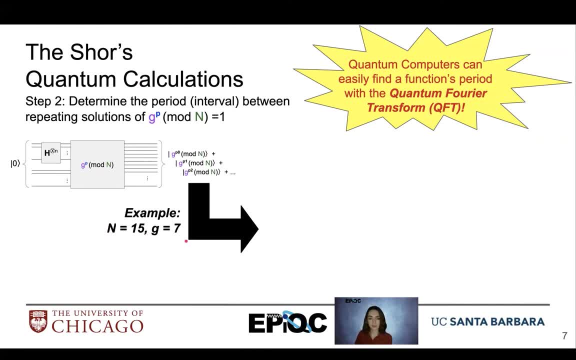 So in this example, for n equal 15 and g equal 7, we can see that we have a plot here of g to the x, g raised to the candidate p values, mod n versus different candidate values for p. so we'll call them x here.